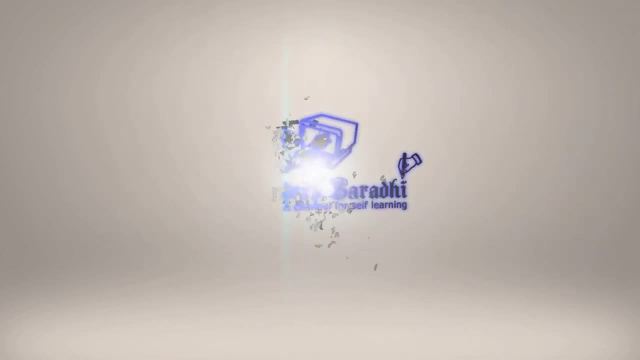 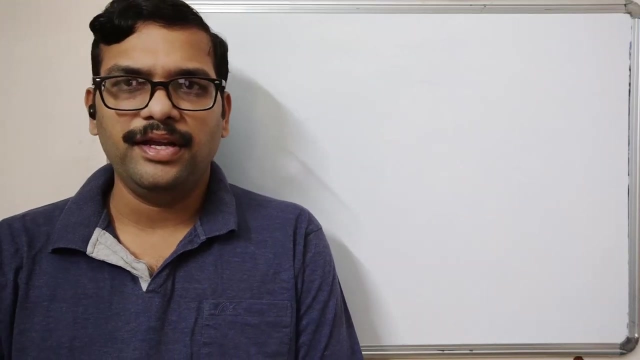 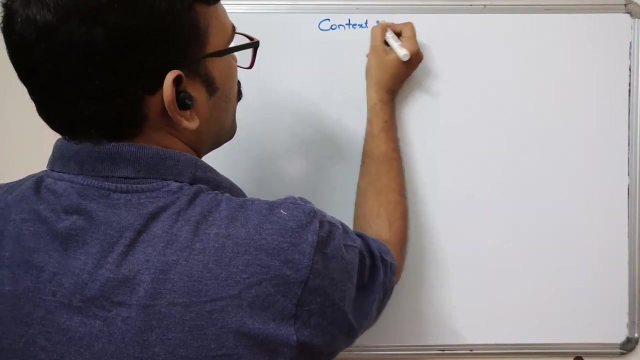 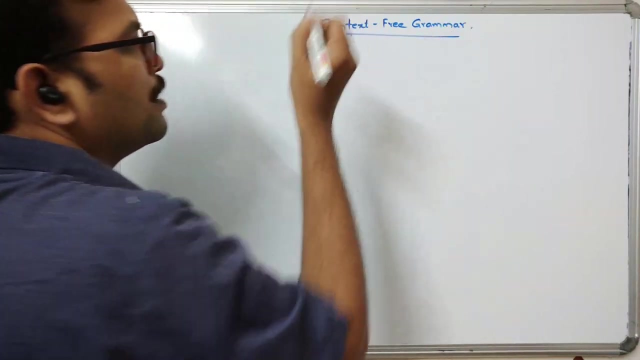 Hello friends, welcome back to our channel. So in today's session we will discuss the context: free grammars in automata theory. Context: free grammar. So in the previous session we have discussed about the grammars. What is meant by grammar and what are the regular grammars. 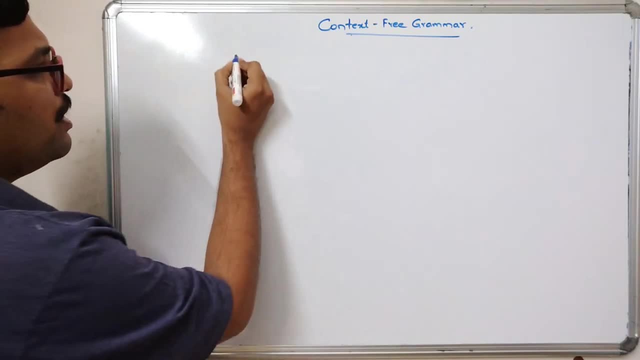 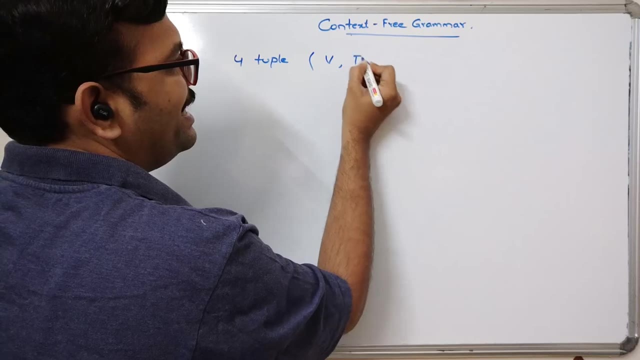 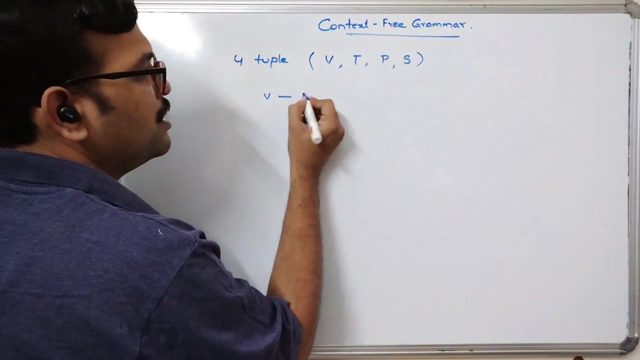 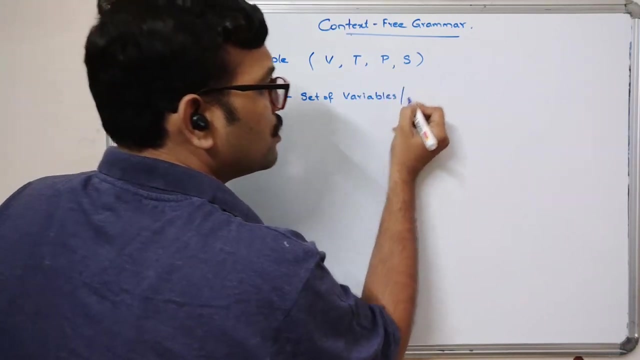 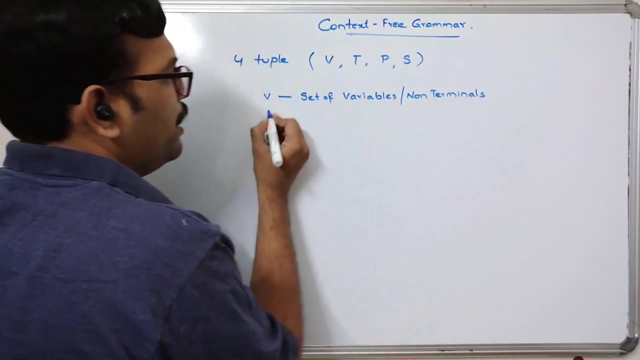 So similarly this context free grammar is also a four tuple or a quadruple. So with V, T, P and S. So we have seen the definition for the grammar. So V means set of variables, set of variables and also we can call it as non-terminals And see next: T is set of. 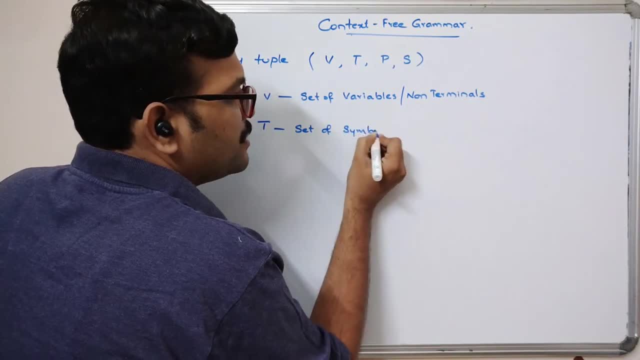 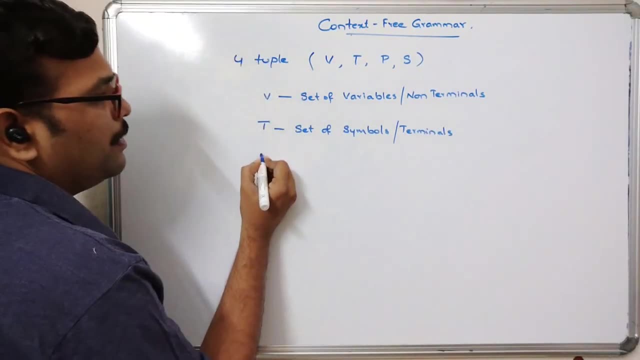 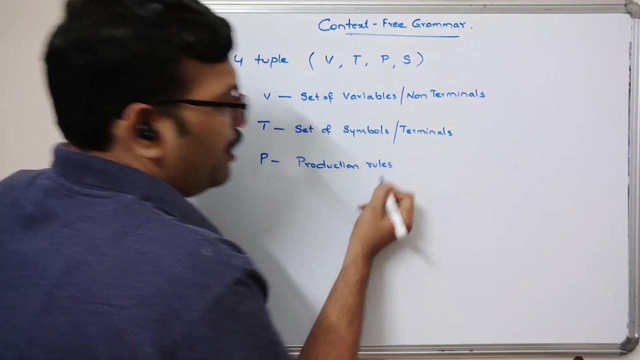 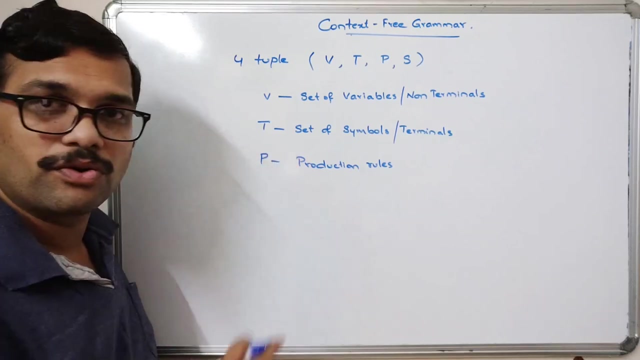 set of symbols. symbols or we can say them as a terminals, terminals- And P is a production rules, is a productions or production rules, And we need to take care about these production rules. So the difference between the grammar and the context- free grammar- is in the production rule. 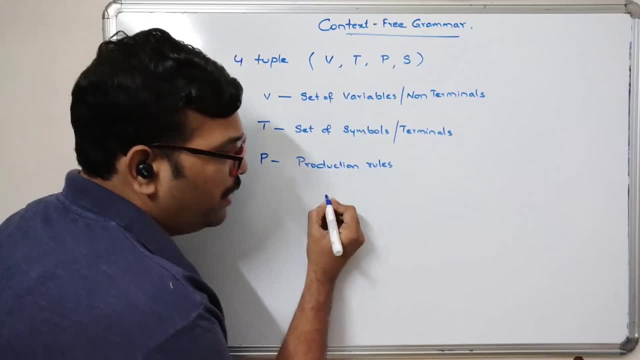 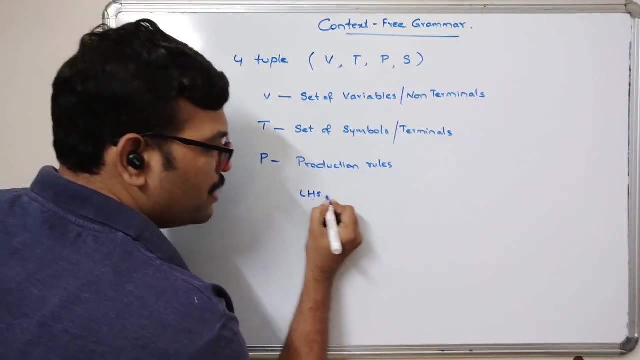 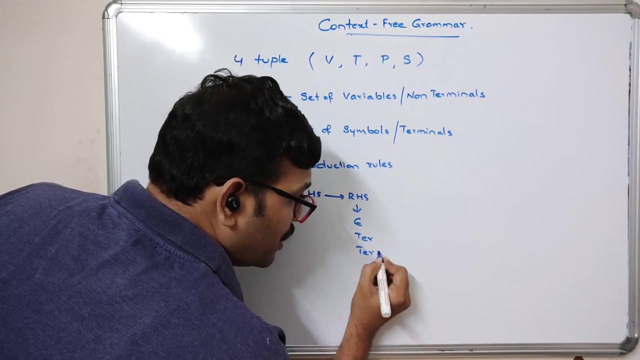 So, coming to the regular grammar we have seen the production should be. So we have seen the left hand side and the right hand side, So the production rules will be defined as a LHS tends to RHS. So on the right hand side that can be epsilon or a terminal, or a terminal with the non-terminal. 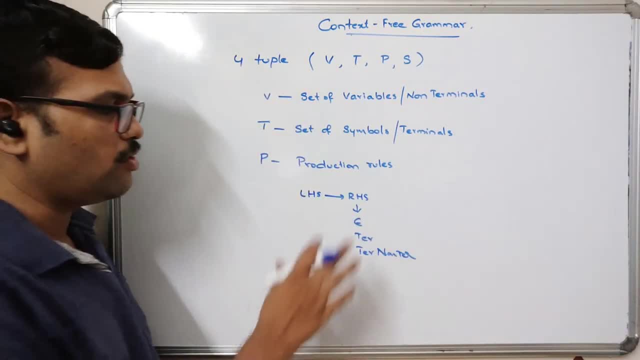 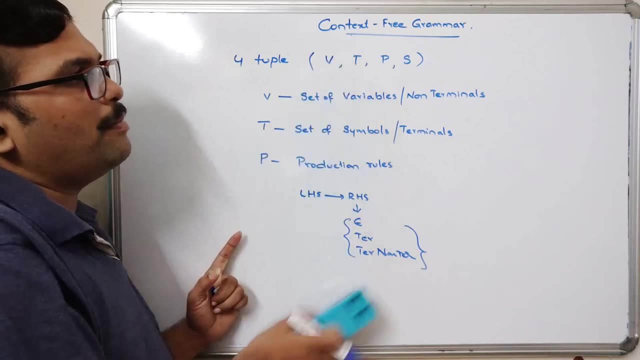 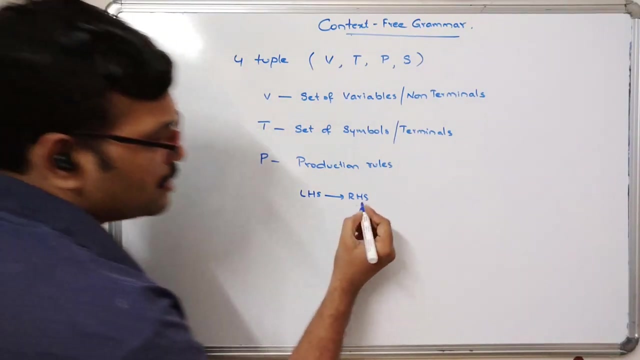 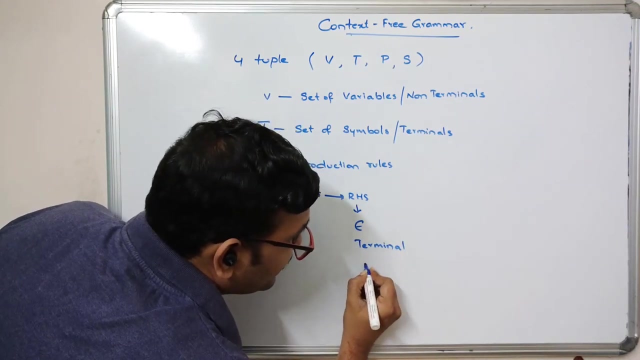 Terminal with non-terminal or non-terminal with terminal. So this is the common rules we need to follow to get the regular grammar. But here the difference over the grammar with the context free grammar is in the production rules: IHS, RHS. in the RHS that can be epsilon or a terminal or string of terminals. in non-terminals, 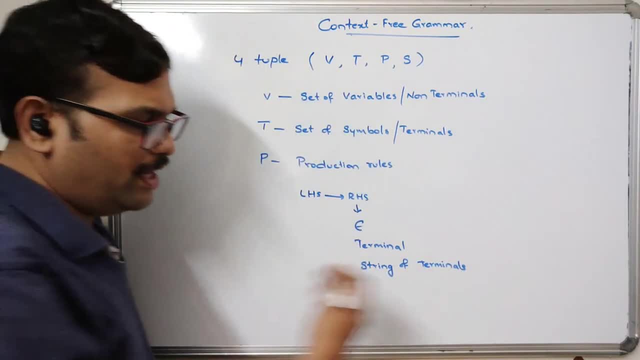 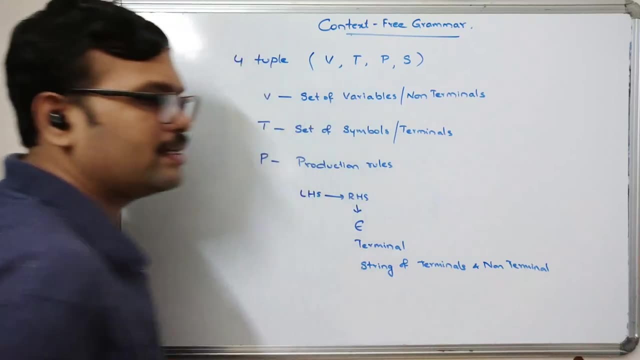 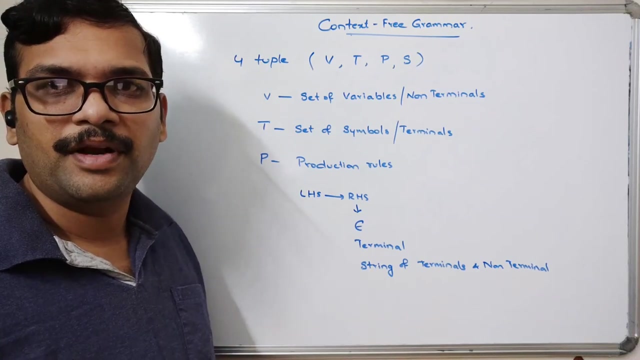 So any number of terminals followed by any number of non-terminals. it can be the combination of terminals and non-terminals. So, but in the regular grammar we have seen there is a restriction that the right hand side should have exactly one terminal and one non-terminal. right. 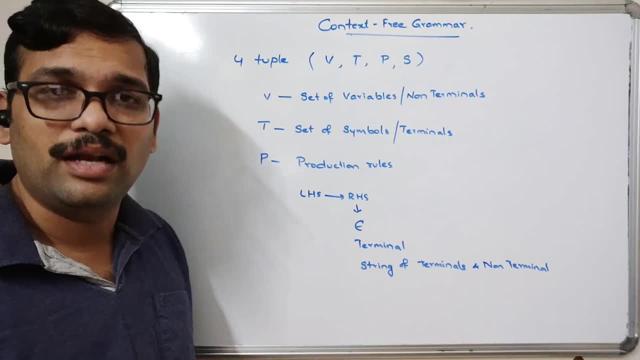 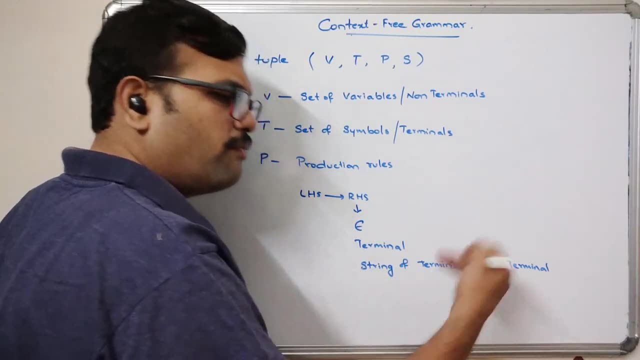 But here there is no constraint upon the number of terminals and number of non-terminals on the right hand side. So if the right hand side can be epsilon or terminal or a string of terminals and non-terminals, So it can be any term, any number of terminals and non-terminals. 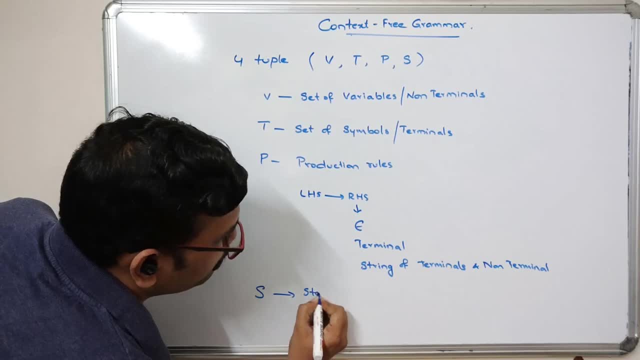 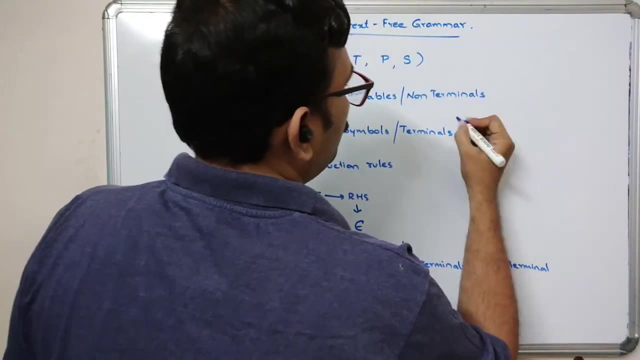 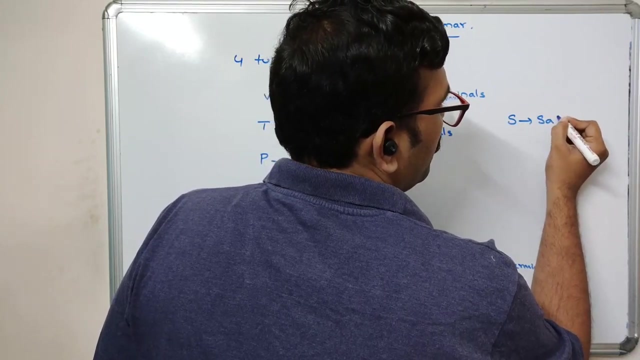 And finally, S is nothing but a start symbol, start symbol right, See for example, for example. So let us take some variables. So let us take the production: S tends to S A A. So this is a valid context-free grammar, okay. 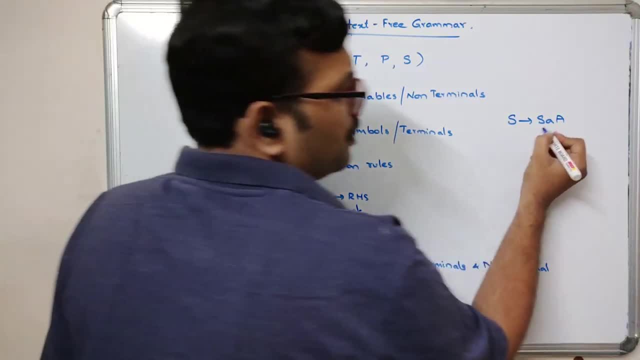 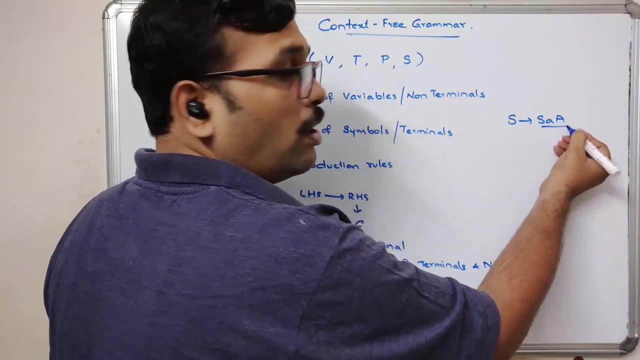 The production is a valid production in the context-free grammar, because so it can be either epsilon or a terminal, or a string of terminals and non-terminals, right? So here we are having one terminal and two non-terminals, one terminal and two non-terminals. 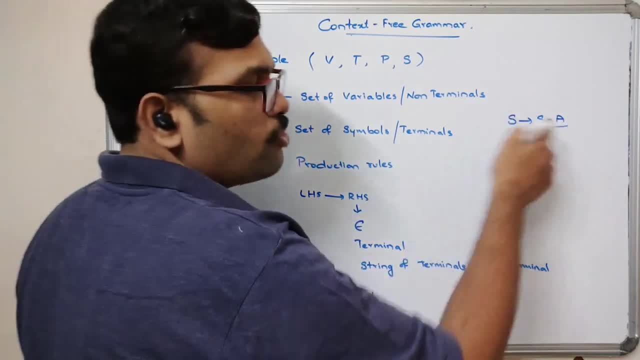 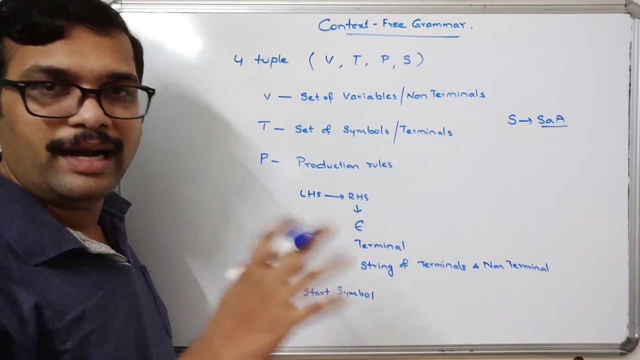 So, even though we call it as a context-free grammar- And this is not- This is not a regular grammar, because if it is a regular grammar, it should have only one terminal and one non-terminal on the right hand side, right, And here also the variables will be represented in the uppercase. 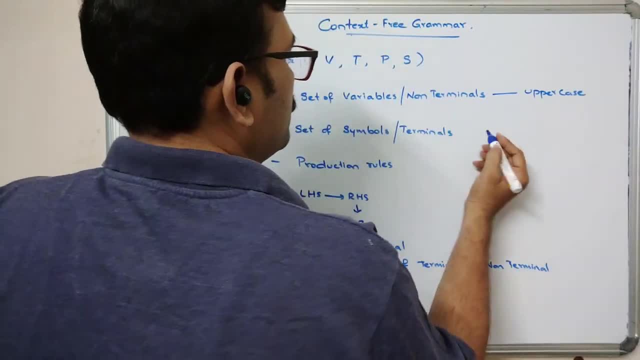 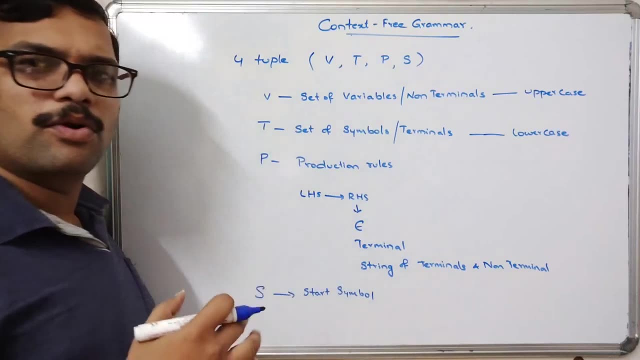 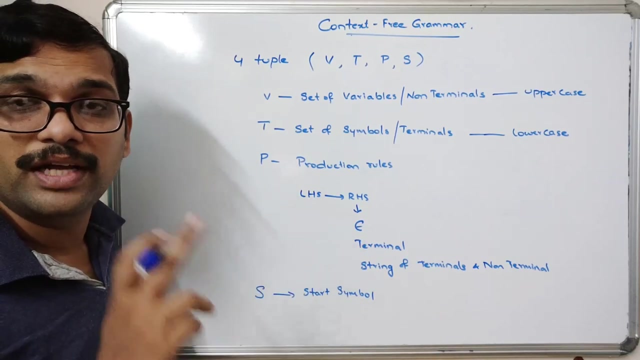 Variables can be represented in uppercase and the symbols or terminals can be represented in lowercase, And from the context-free grammar also we can derive the strings which accept this grammar. So here the string means a set of terminals. So a string should not contain a non-terminal. 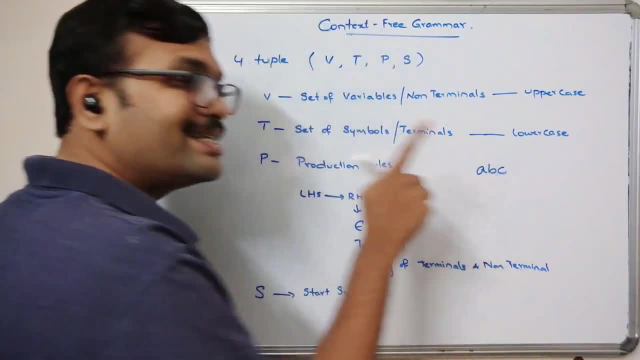 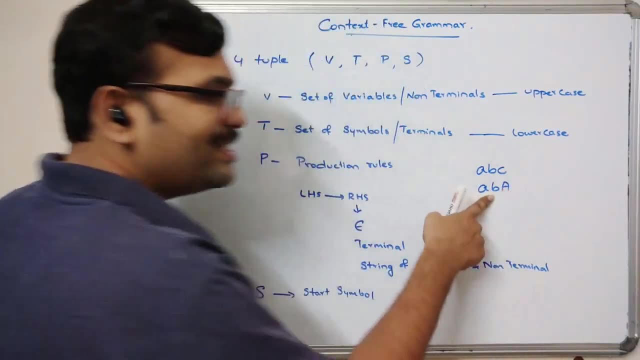 So, for example, so if it is A, B, C, this is a string. okay, This is a string because everything is a non-terminal. And if the string is like this, so this is not a string. okay, Because here we are having the non-terminal, okay. 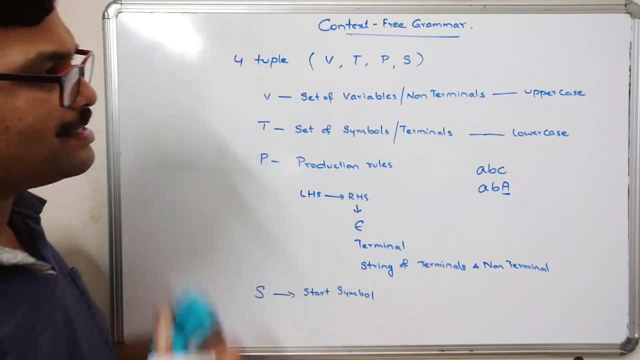 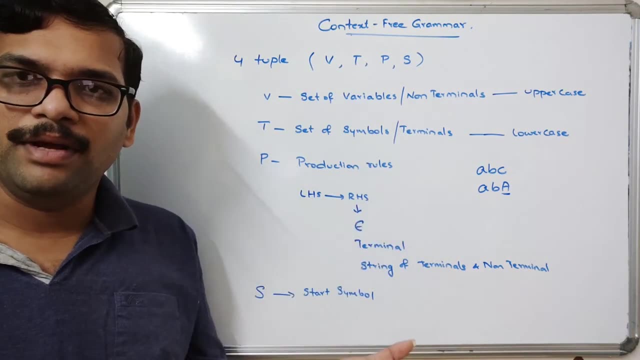 So string does not contain the non-terminal. So we can construct or we can derive the strings which accepts the following grammars: okay, So we need to write the grammar And we can derive the strings which accepts the grammar. So we will see one example on this context-free grammar. right? 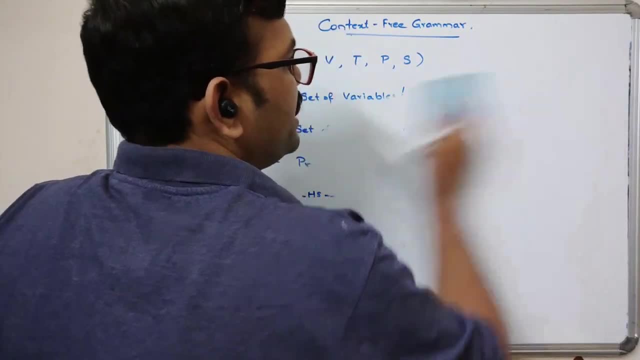 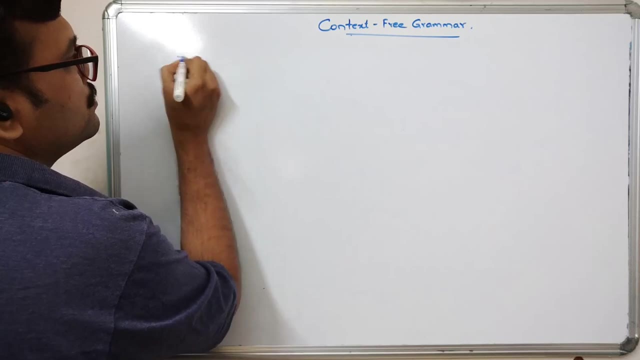 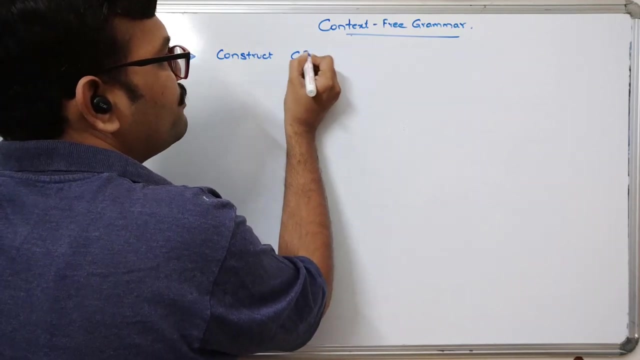 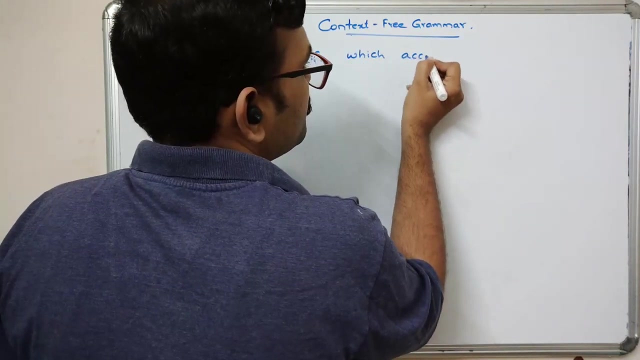 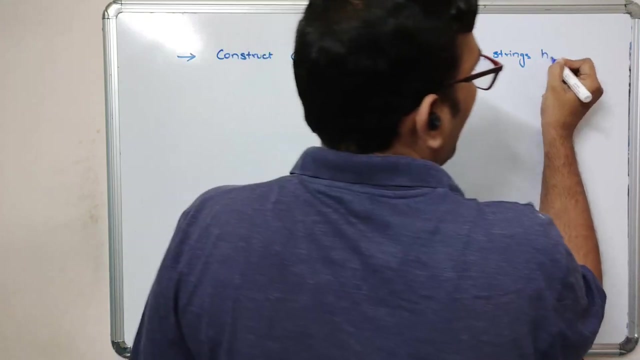 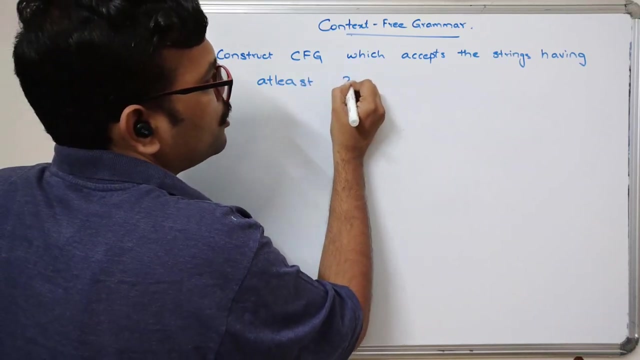 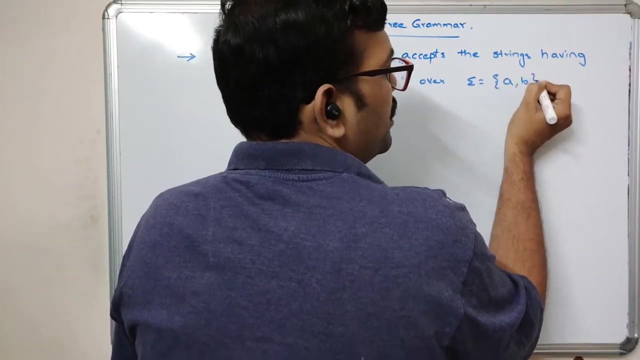 So let us take an example for this one: See Construct CFG. CFG means context-free grammar Which accepts the strings having at least two A's over alphabet A- B. So we need to write the context-free grammar for this particular condition. 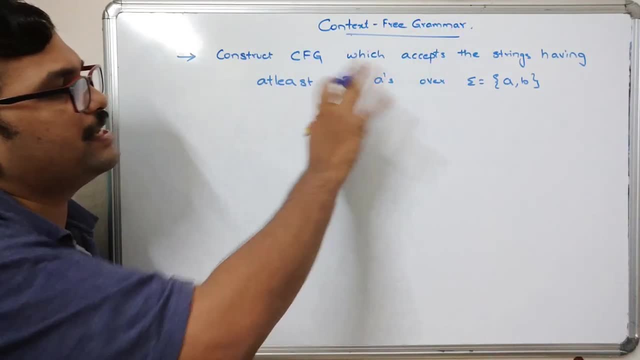 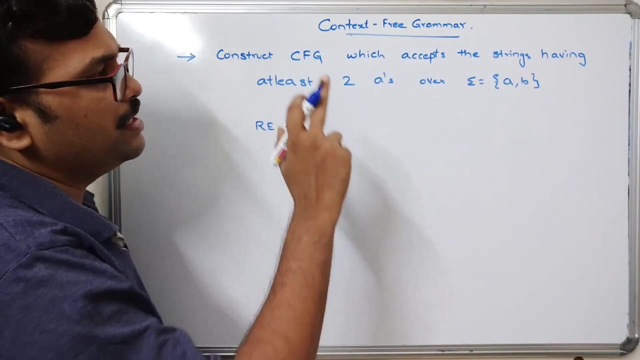 That means We are writing the context-free grammar which accepts all the strings having at least two A's. So first of all we can write the regular expression. We can write the regular expression. So here the question is, we have to, I mean, construct the grammar such that the strings 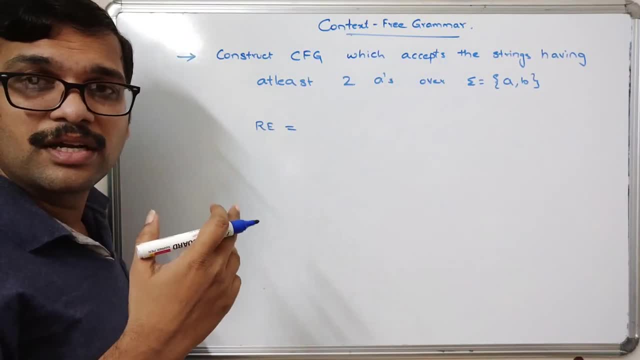 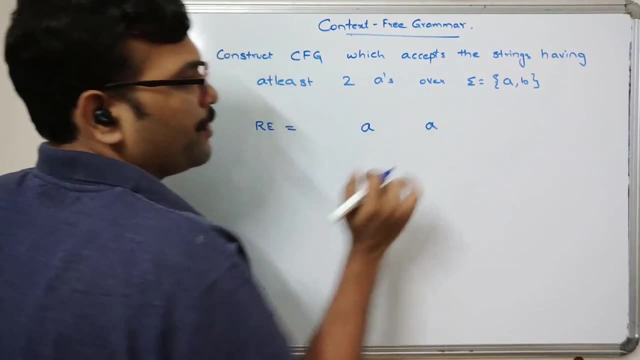 the strings having at least two A's, at least two A's, So it is not a consecutive A's Anywhere it can be. So I will write A and A. okay, So it can start with A or B. 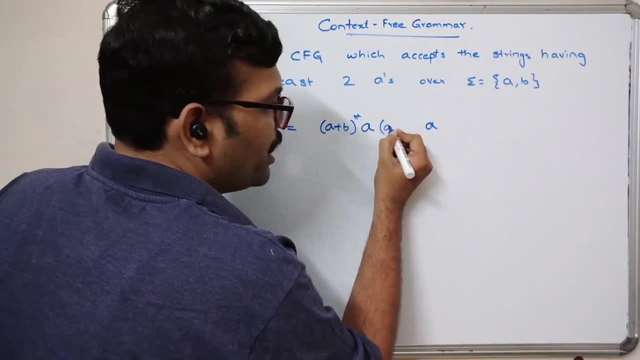 Any number of A's and any number of B's. In the middle we can have any number of A's and any number of B's. In next here we can have any number of A's and any number of B's. right. 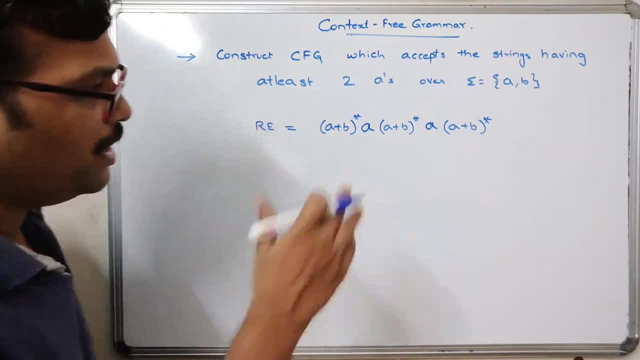 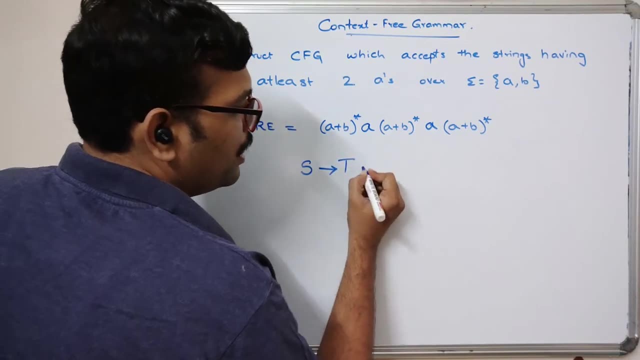 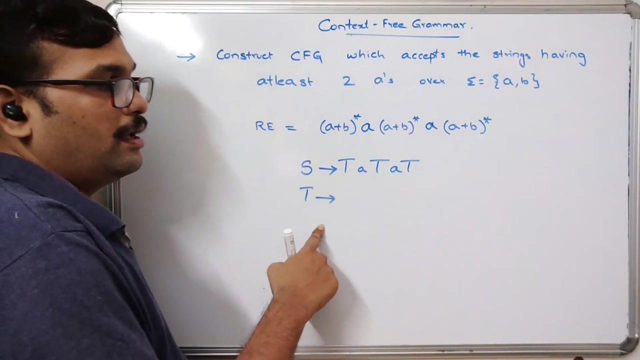 So in between there should be exactly A's. So here we can write the context-free grammar as: take one non-terminal and consider this one as another non-terminal: A, T, A, T. Now T can be, T can be any number of A's and B's, right. 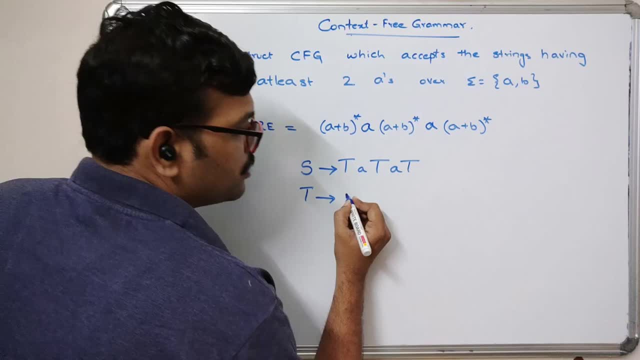 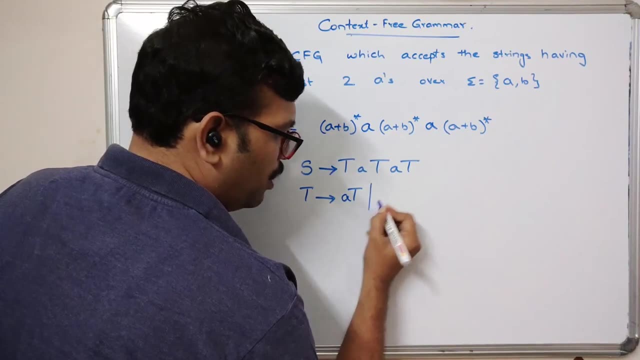 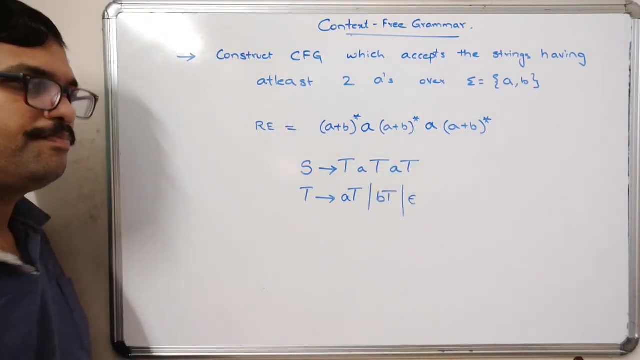 Any number of A's and B's. So for example, if T, T can be any number of A's or any number of B's, or epsilon null, epsilon null. So here this we can repeatedly, we can apply this one right. 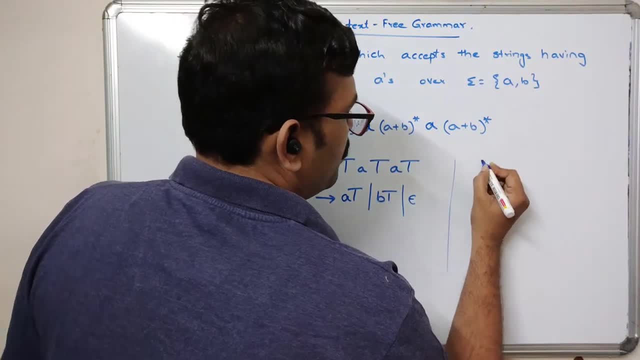 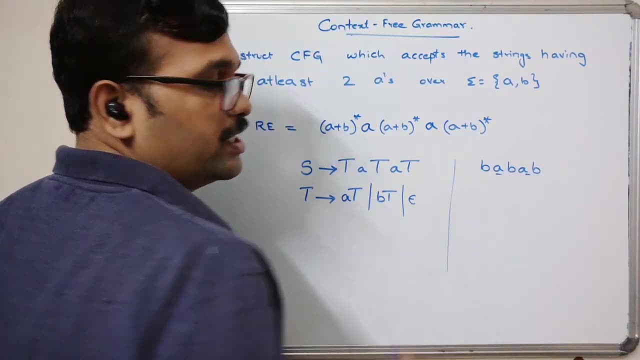 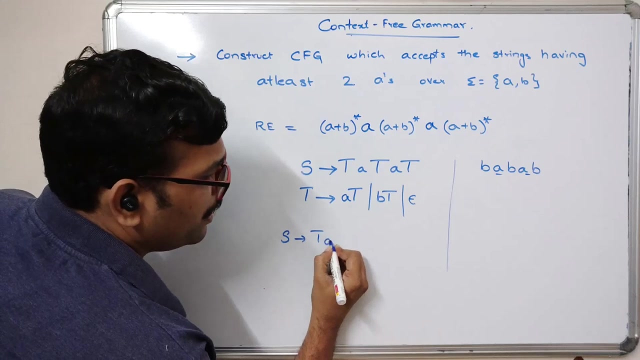 So, for example- let us take one example- So let it be B A, B. Okay, So in between there are two A's, right, So this is a valid string. So now you can consider: from this S, S can be T, A, T, A, T, and now this T can be replaced. 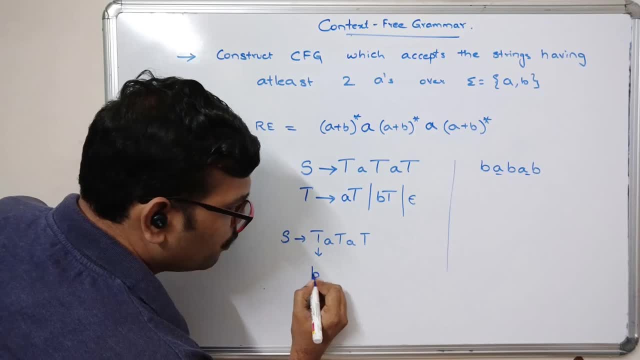 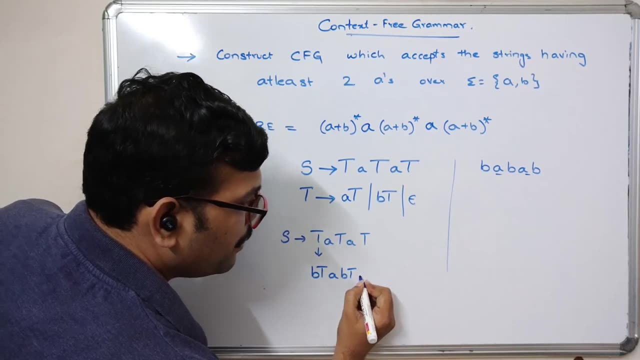 with B T Okay, Because it should start with this one, So B T A and this one also can be replaced with B T Okay. A T A B. Okay, So we can consider these two right. 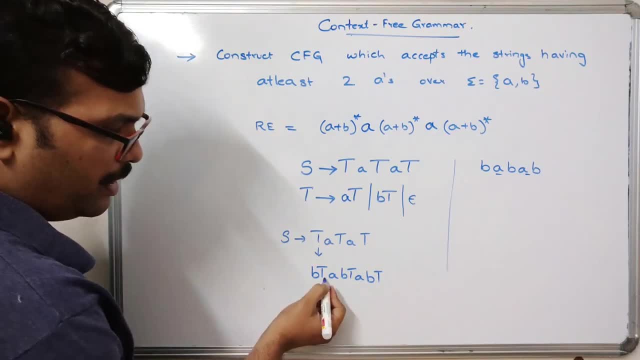 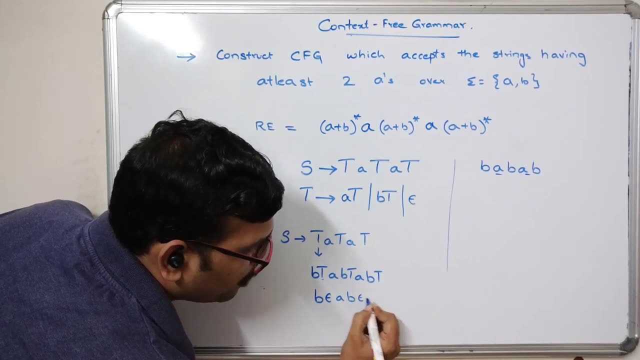 And again we can replace with B T. Now you can observe here: here T can be replaced with epsilon, So B, epsilon A B, epsilon A B, So epsilon. you can remove this one. 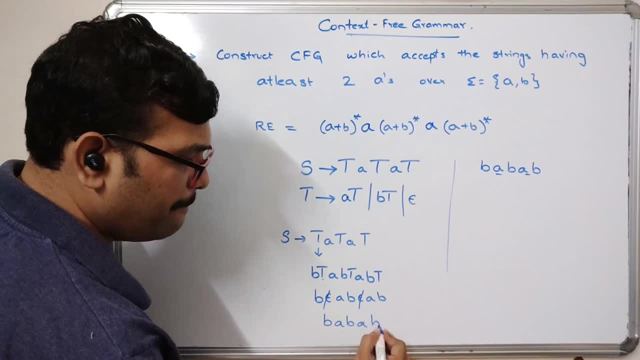 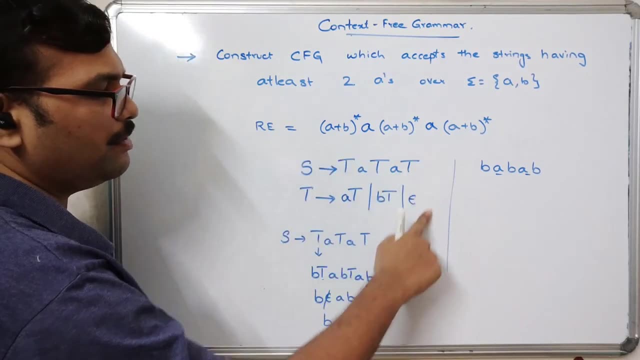 So it will be B A, B, A B. so which is as K, right? So hope you understood. So you have to construct the context free grammar such that it should accept the say A, B, A B. 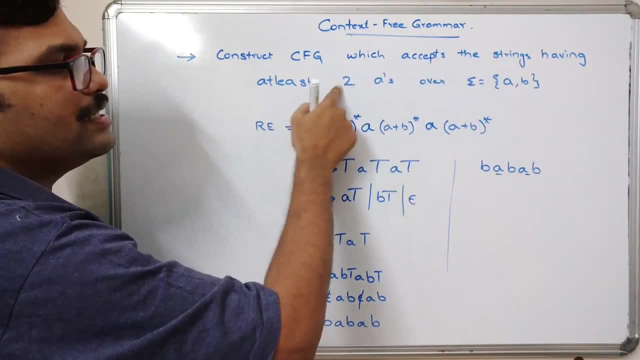 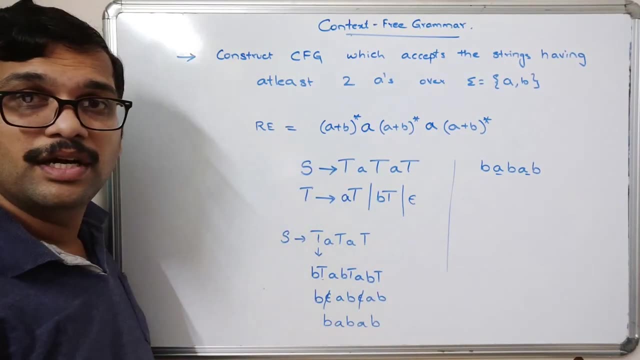 Okay, all the strings which are having at least two years. So it would be very easy for you if you write the regular language first, sorry, regular expression first. So if you write the regular expression from that regular expression, it is very simple to write the context-free grammar. 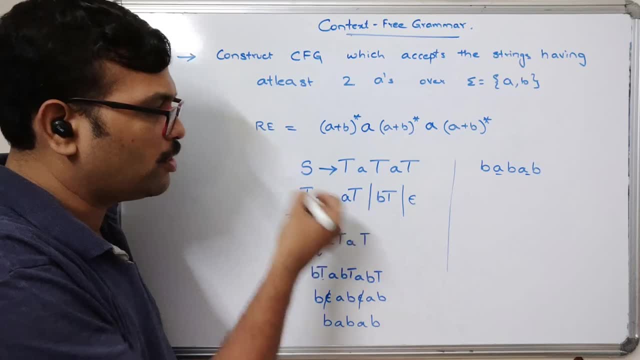 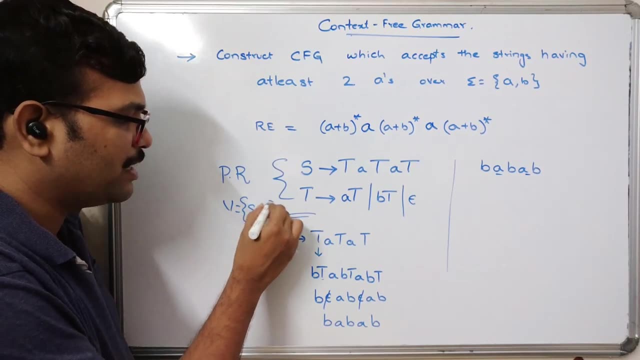 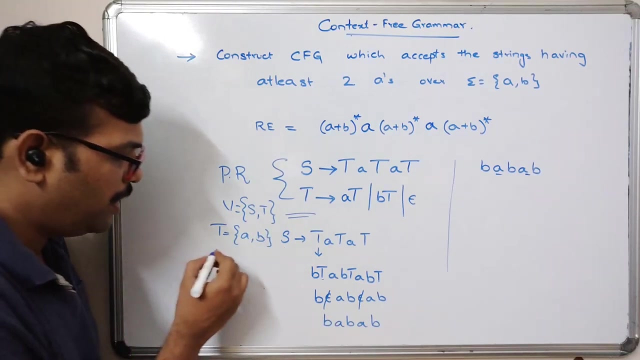 right. So we are supposed to write the production rules, and these are the production rules. these are the production rules. and V is nothing but S and T, those are non-tangles, and T is nothing but A and B, which are nothing but symbols, and S is a start symbol, which is nothing but S. 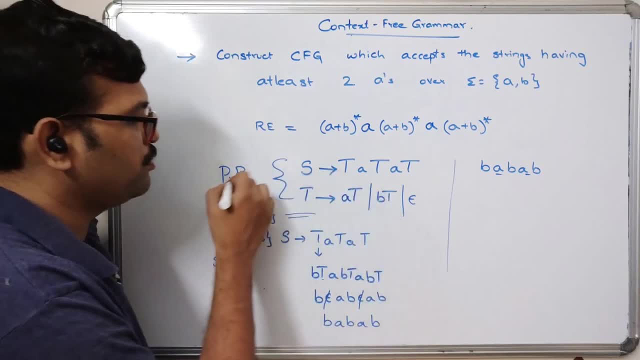 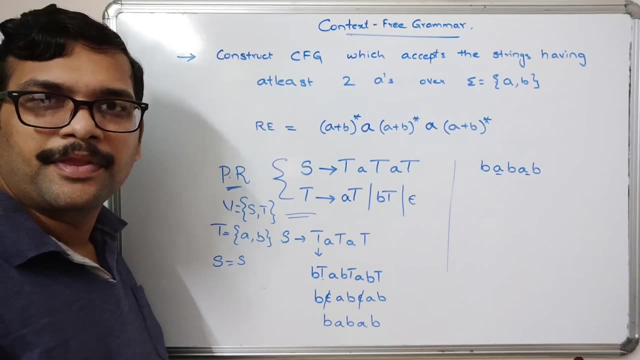 here, right, And these are the production rules. these are the production rules. So, like this, we have to construct the context-free grammar right. So hope you understood this one. and the only rule is that we have to construct the context-free grammar right. So hope you. 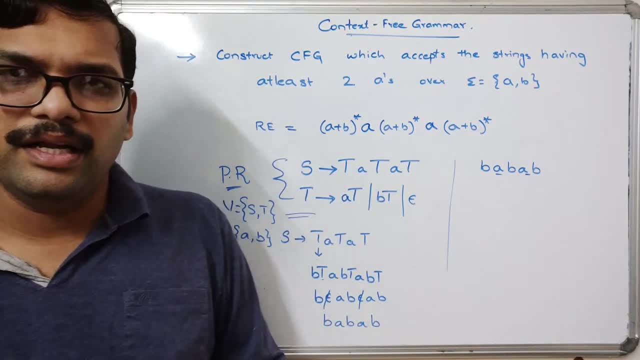 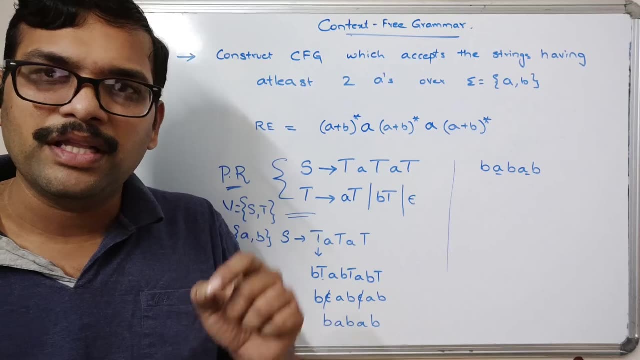 understood this one, and the only difference between the regular grammar and the context-free grammar is on the production rule. So in the production rule on the left right hand side, if it is a regular grammar, there should be one non-terminal followed by one terminal or one.